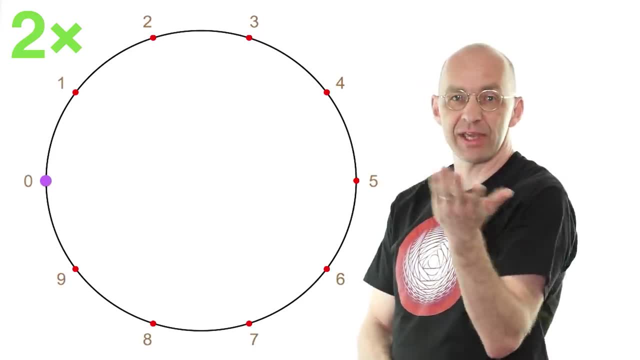 So 2 times 0 is 0. So 0 is the same thing. so we don't do anything, Okay. 2 times 1 is 2.. 2, okay. So we connect the 1 to the 2.. 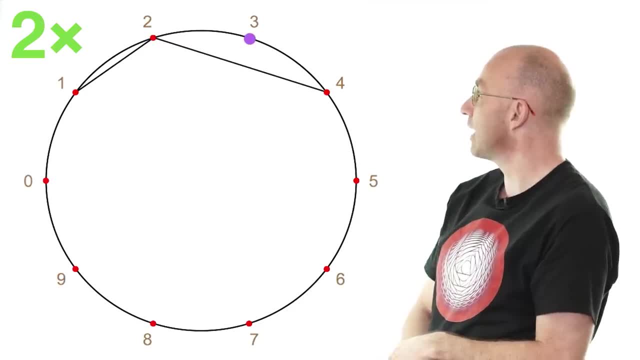 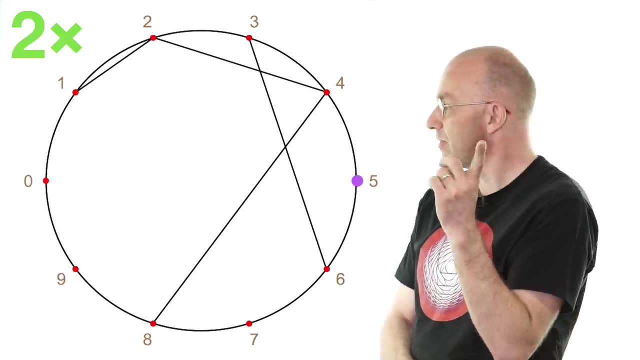 Then 2 times 2 is 4.. Okay, so we do this and we keep on going. Pretty obvious Now 5.. 2 times 5 is 10.. 10. Remember, 10 is also over there, so we connect that guy up. 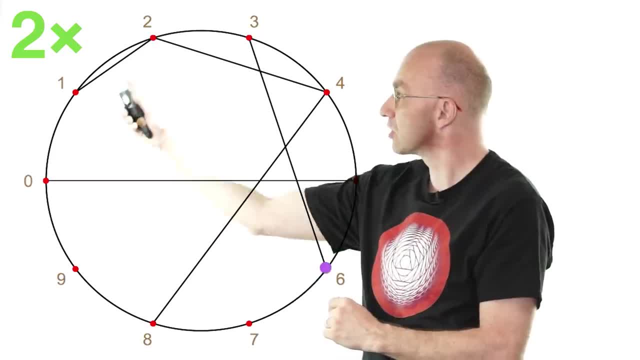 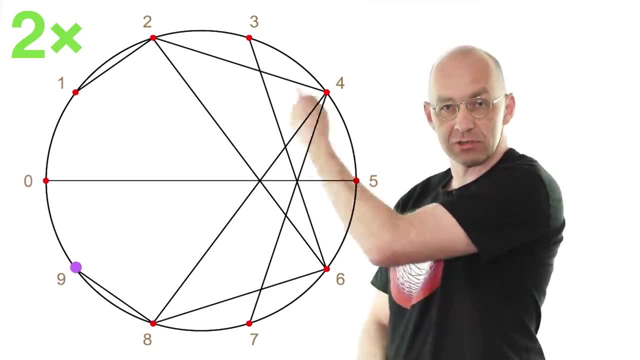 And then 2 times 6 is 12,, which is also the 2, so we connect that one and then kind of just keep on going like this, okay, And then you're at 9, and you've pretty much. 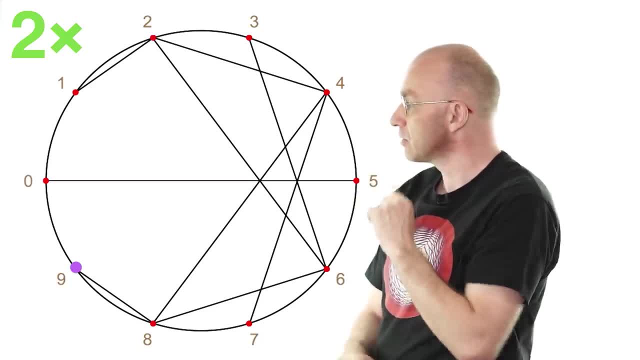 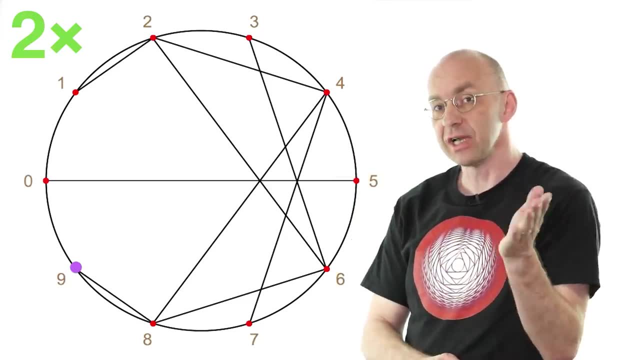 gone all the way around. Now you could go on. so, for example, we could now do 2 times 10, and 2 times 11, and 2 times 12, and draw in those connections, but actually the connections are going to be: 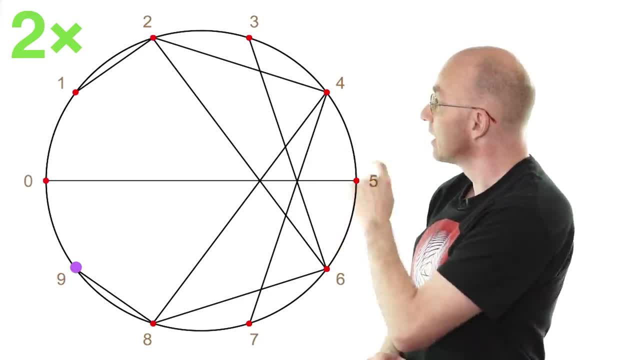 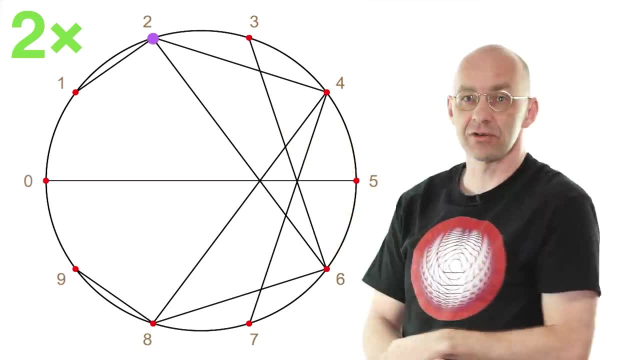 exactly the ones that we've already drawn, which we can actually stop here. Just to illustrate, let's just go up to 2.. 2 times 12 is 24.. 24, which corresponds to the Four. Four, and that connection's already there, right? 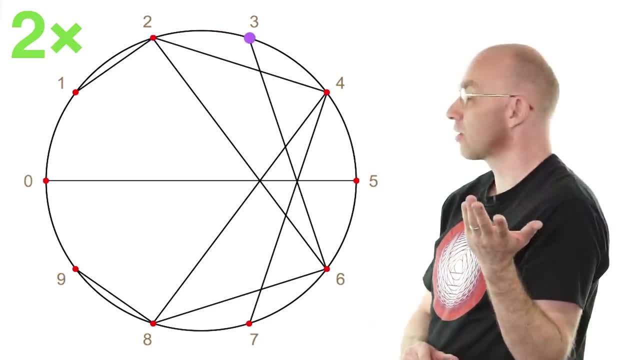 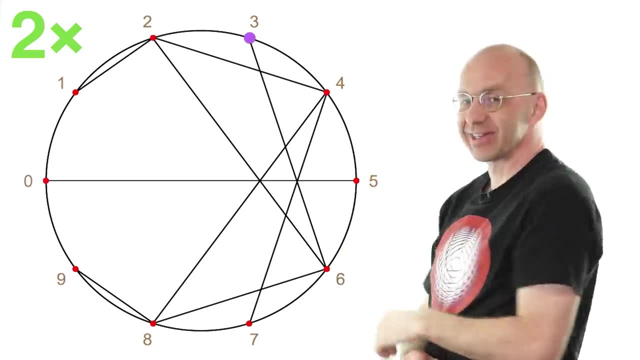 And 2 times 13 is 36.. Not quite 2 times sorry. what? 2 times 13.. 2 times 13,, 26.. 26, and we've already got the six. Of course, we made a choice there at the beginning. 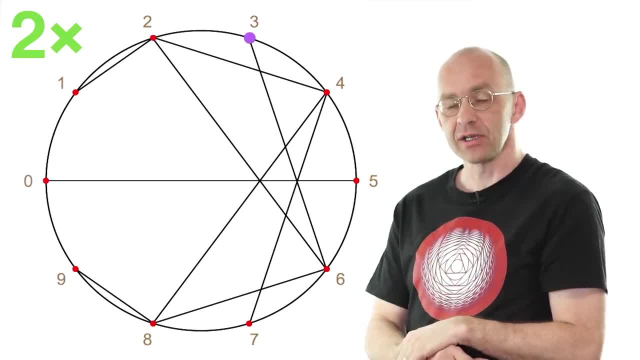 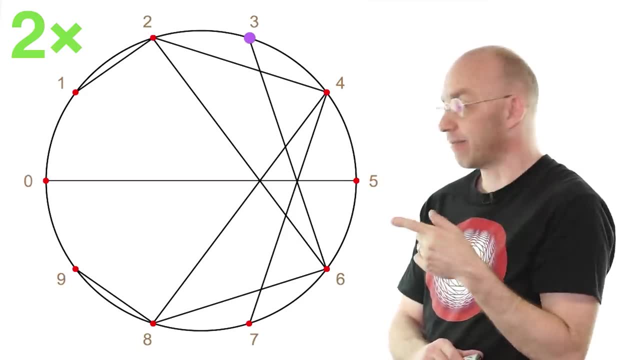 that 10, right. If you change that 10 to anything else, well, the picture changes, but pretty much everything I said stays the same. okay, So, for example, if you switch from 10 to 11, we get this guy here, you know. 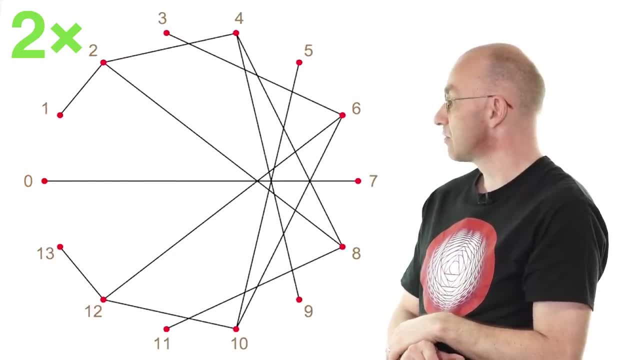 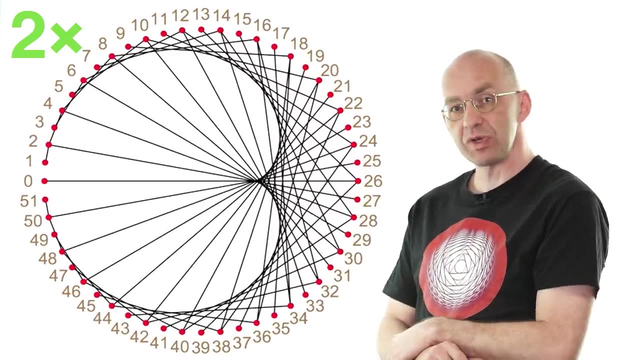 and then 2 times 12,, 12,, 13,, 14,, 15, and let's just see what happens. Hmm, pretty nice. So quick question: Yeah, All these pictures that you're showing, it seems that they are symmetric. 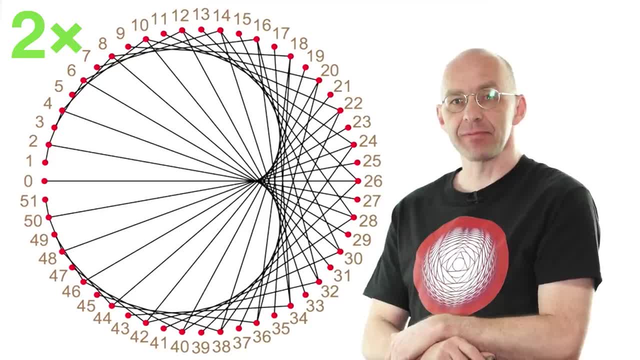 Yep In the horizontal axis. That's right. yep, yep, yep, yep, yep, yep. Is that for a particular reason? Yep, there's a reason, and actually let's just give this as homework. 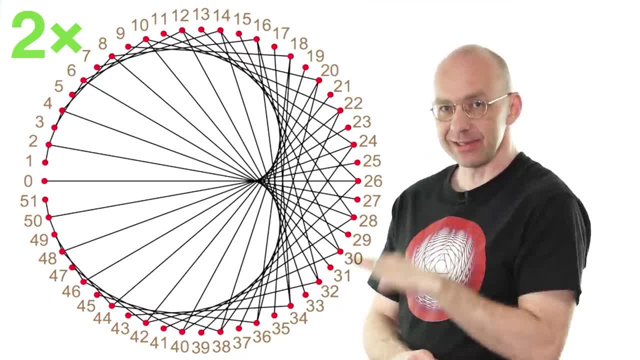 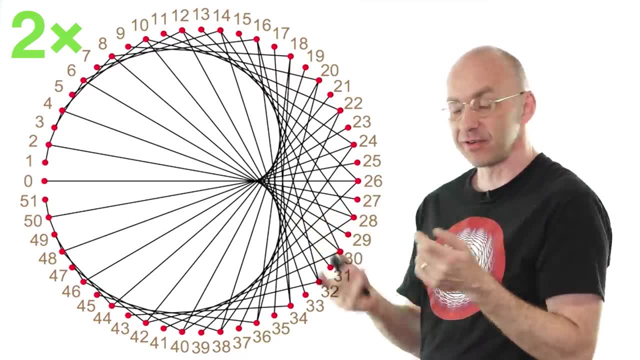 for our guys here to figure out In the comments. tell us why there's a symmetry. Of course, what's much more interesting here is that curve that somehow magically materializes when you kind of up the number that you choose at the beginning. okay, 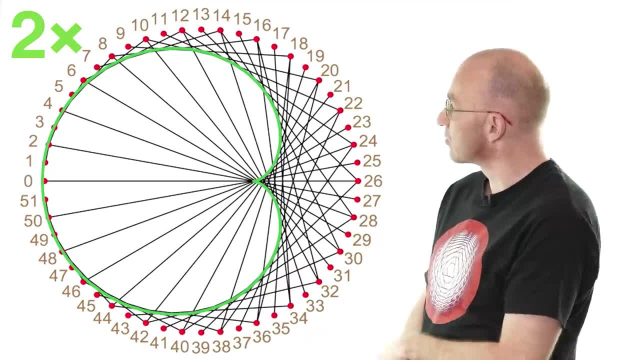 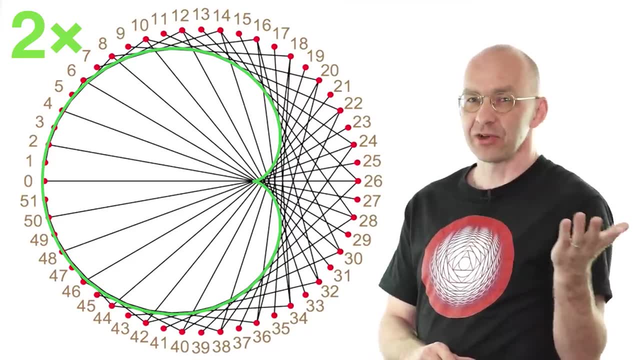 And actually I'll just highlight it a bit. So there's this strange curve here and it's actually got a name. It pops up all over mathematics. It's called a cardioid. Like in cardiology, this means heart, okay. 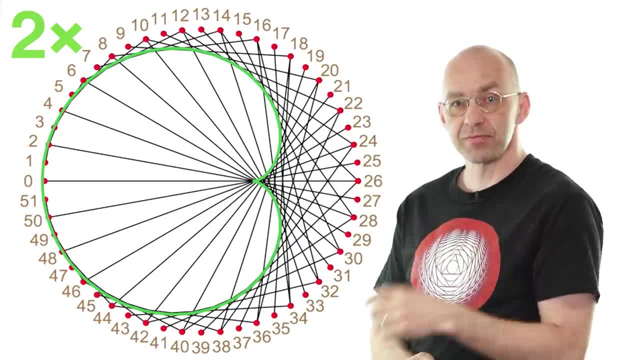 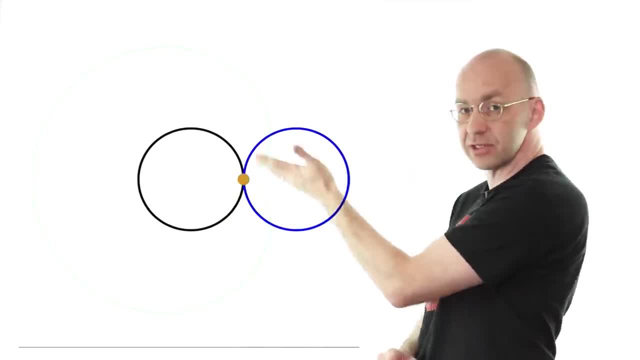 So it's like a heart curve, mathematical heart curve, and it comes up in all kinds of places and I'll just show you a few. okay, So, for example, you can have it as a rolling curve. You roll one circle around another circle. 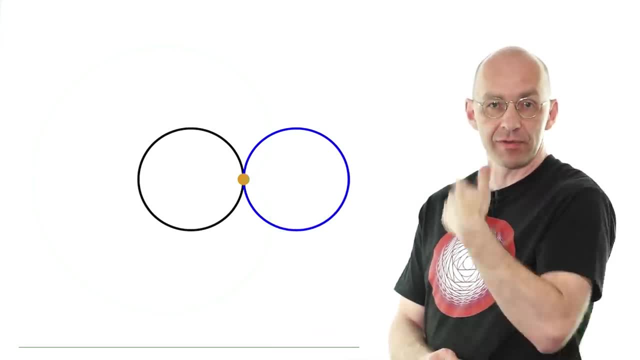 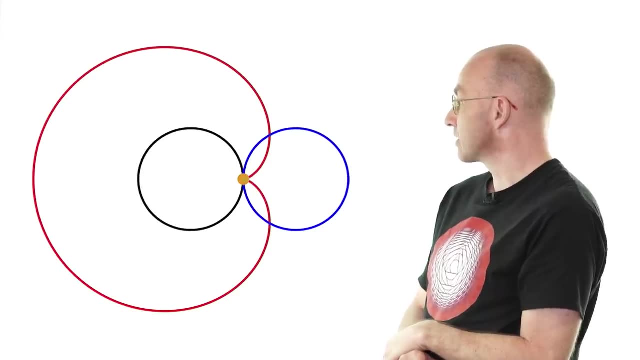 and just see what happens to one of the points on the boundary of the rolling circle. okay, So, from over here, and what it does is it traces the cardioid. okay, Now, where else can you see it? Well, sometimes you can see it in your coffee cup. 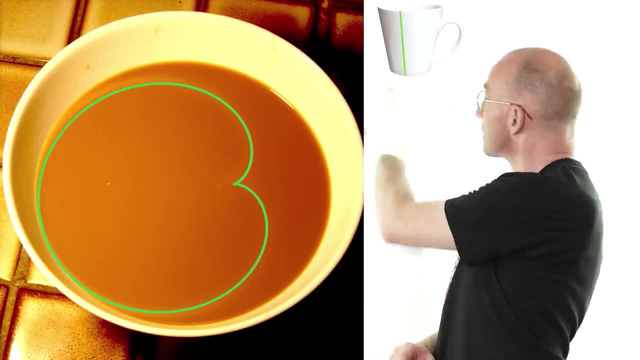 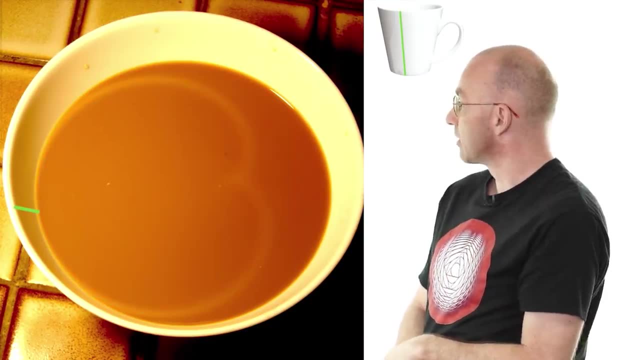 If you've got a conical coffee cup like this and the sun is in the direction of one of those green lines in the coffee cup, then you can also see a cardioid in there. Where else? Well, there, right there. 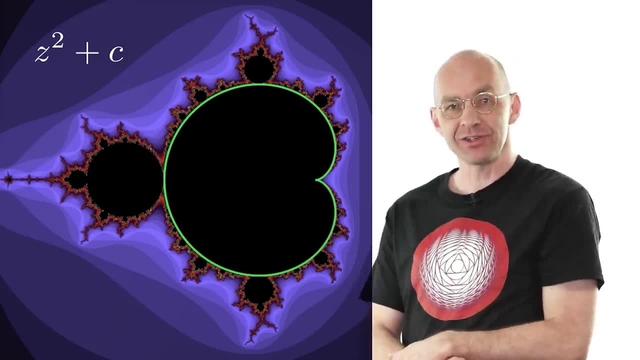 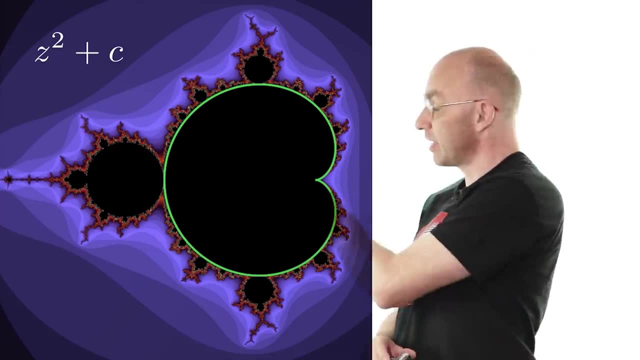 in the Mandelbrot set. So the biggest bulb in the Mandelbrot set is a cardioid. The second one is actually a perfect circle. Now, this would be a good one to figure out. why is this guy a cardioid? 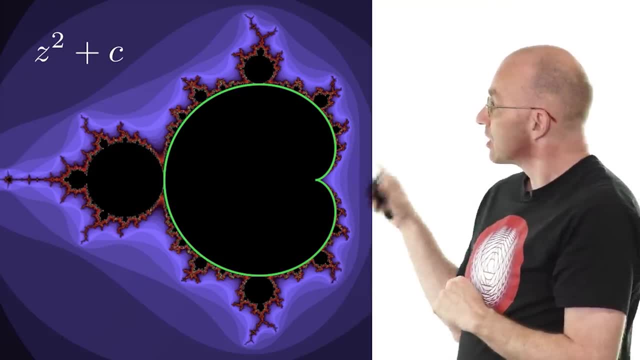 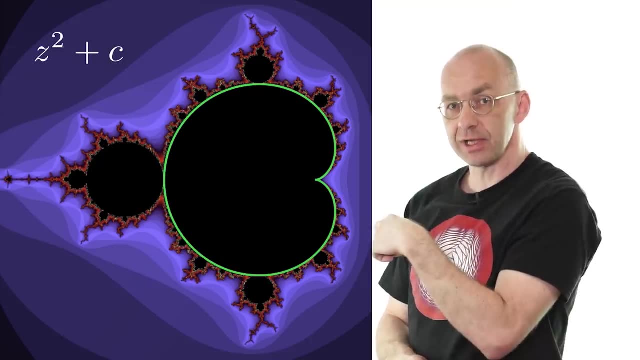 So I'm just gonna trace this down somewhere Now, just for those people who know something about this stuff. that's the equation that we use to make up the Mandelbrot set, and there's a two in there. okay, So that's important. 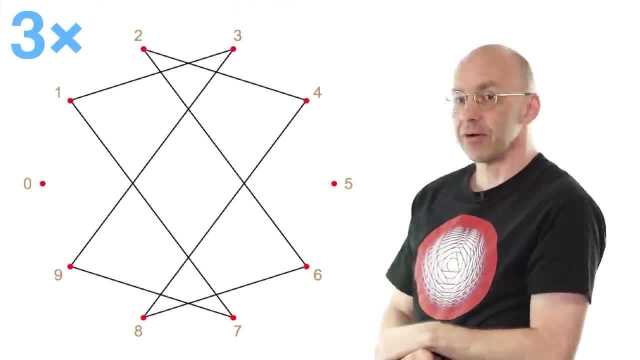 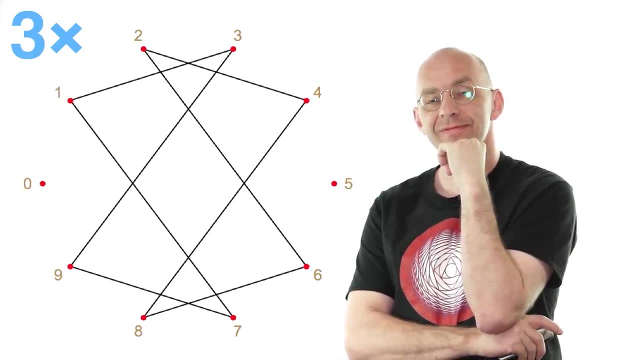 We just had the two times table, so let's just keep going, okay, Now, yeah, If you want one more thing about the cardioid shape, is that actually, as a video producer, I know that. microphones- there is a category. 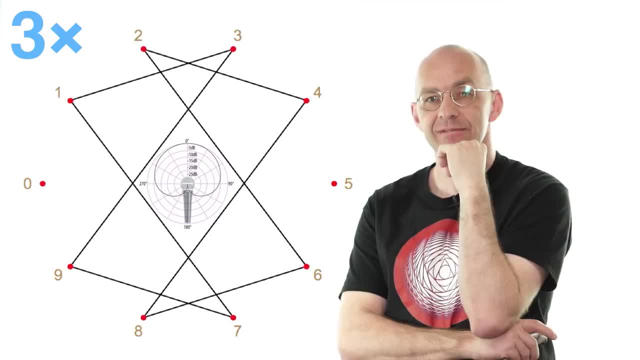 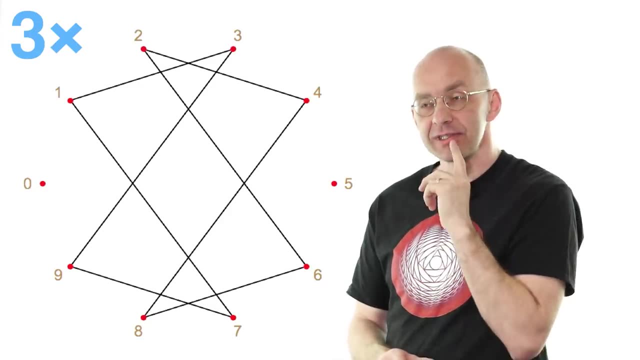 of microphones called cardioid microphones, and that's because they pick up the sound in that area from that direction. Okay, right, well, maybe we do another video on this. Okay, now we can also, instead of doing the two times table. 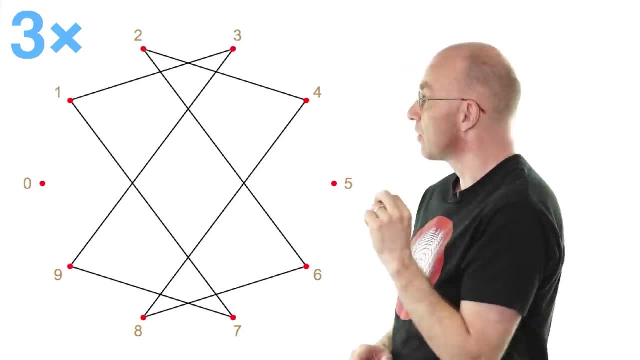 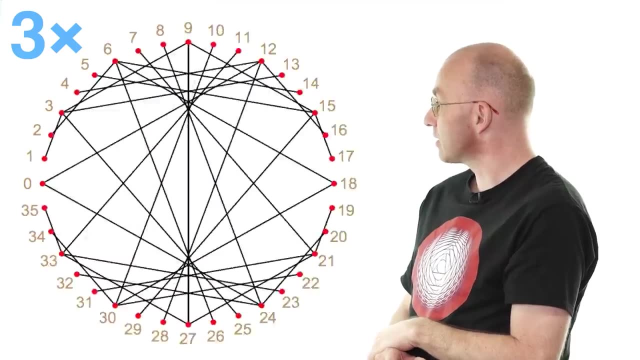 we can do the three times table. And if you do the three times table, well, what we get is this pattern here for initial choice, which is 10, and then I'll just you know up the numbers there. and what do we get? 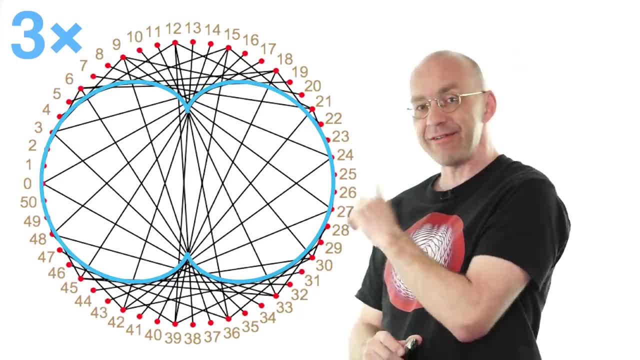 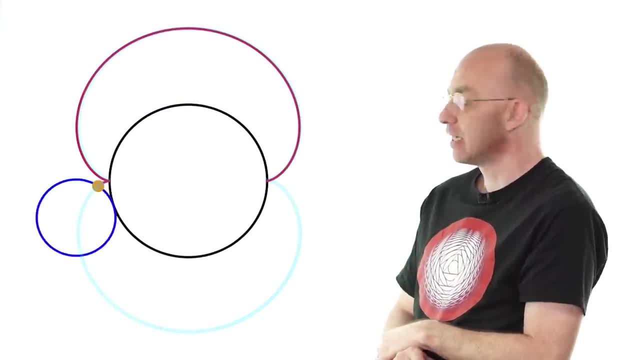 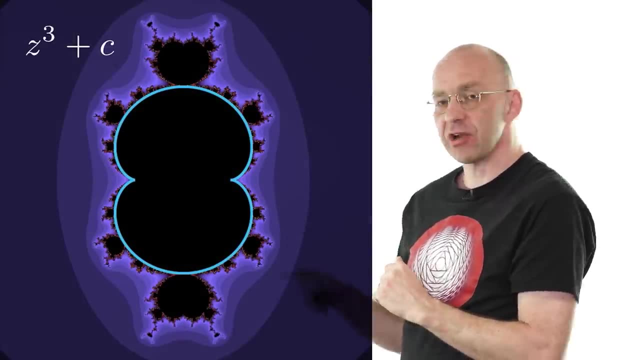 Woo, another curve. Another very famous curve is called the nephroid, which is kidney, you know, Okay, whereas this one also has a rolling curve here, the circle that rolls is half the size of the one that is rolling around. It's also in a generalized Mandelbrot set. 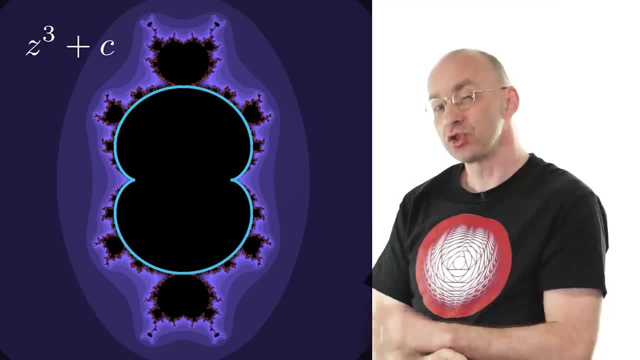 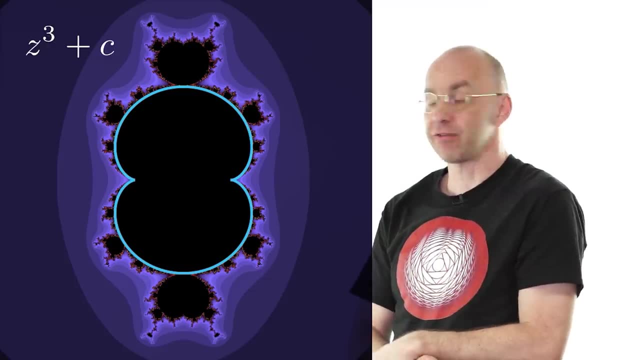 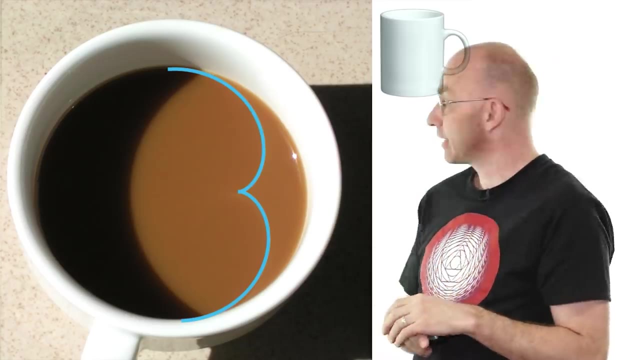 so remember before we had an exponent two. here we're talking about three times table. we change the exponent to three and you actually get the main bulb here being the nephroid. Okay, we also get it in a coffee cup. This time we need a like a straight coffee cup. 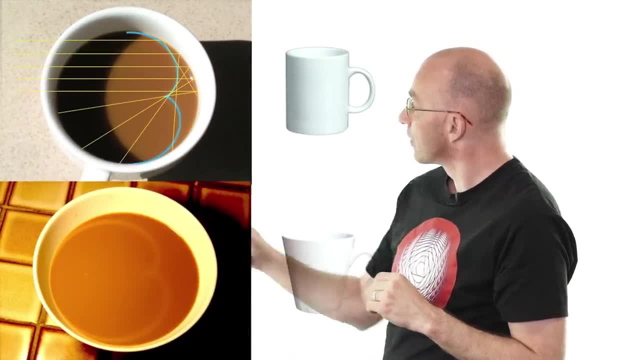 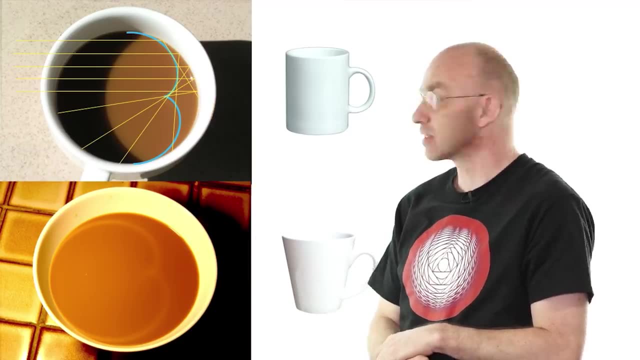 and the light rays kind of come in like from one side. Okay, so they kind of come in straight, like this, and then they kind of bounce around inside the cup and make up this curve. actually, you know this way of making up a curve. 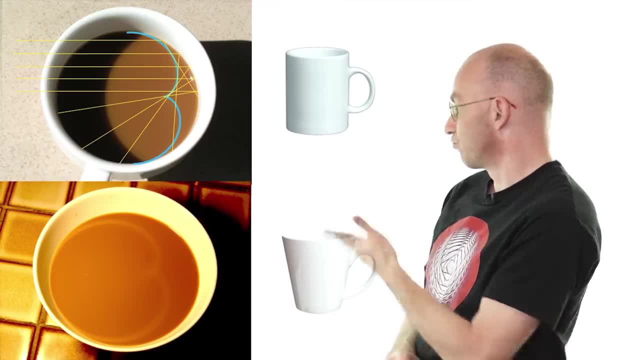 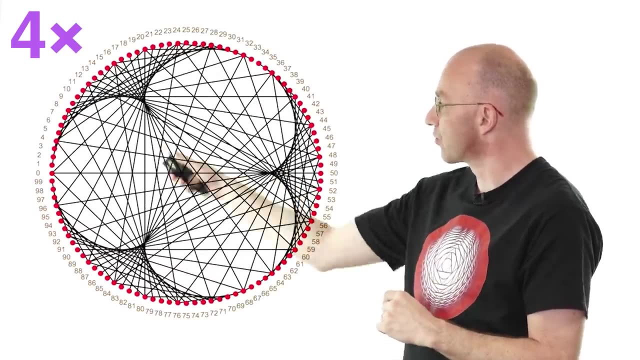 It's called a catechostic in mathematics. So there we go. what else have we got? Four times, and you can see kind of see a pattern now. you know, four times gets you three, three petals before we had. you know three times two petals. 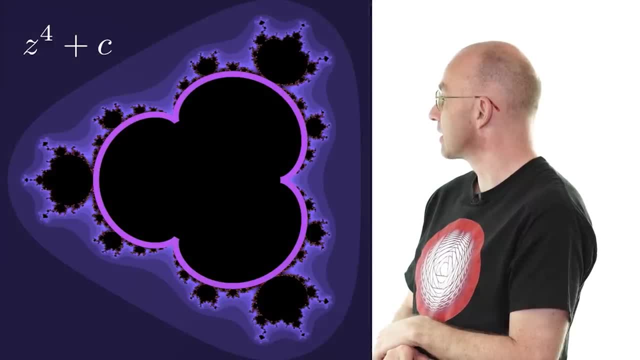 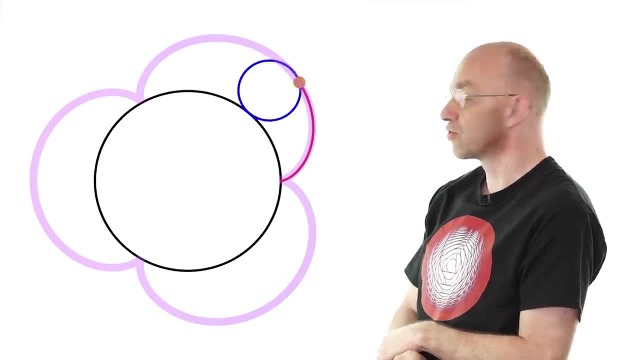 Okay, and then all these other things that we've kind of been highlighting here. they work. two, there you know, exponents gone up to four. this is the generalized Mandelbrot set here, and we've got the rolling curve happening again, right. 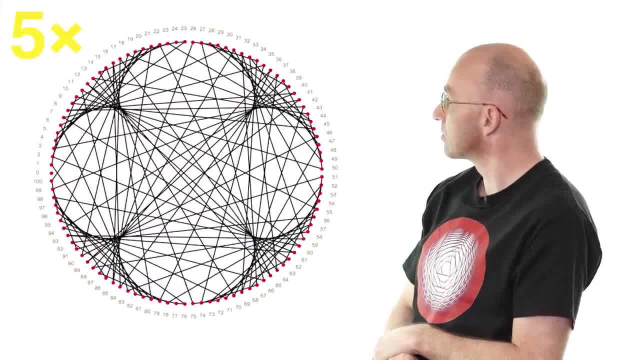 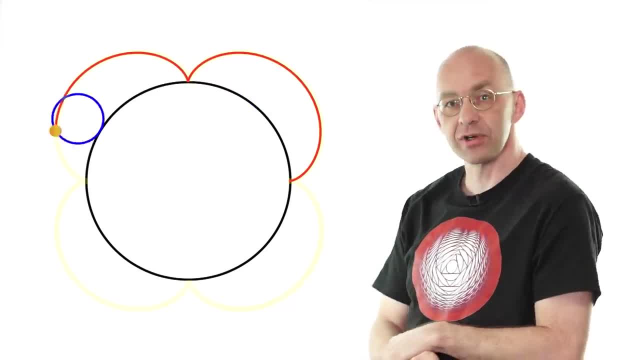 And then, just for good measure, just one more guy here, that's the five, that gets four petals, and we've got the Mandelbrot set here and we've got the rolling curve. So all very, very neat, okay. 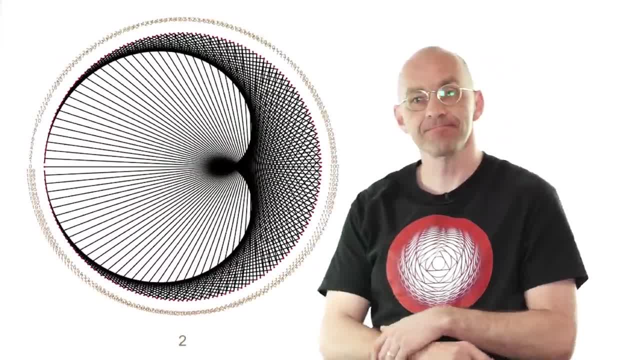 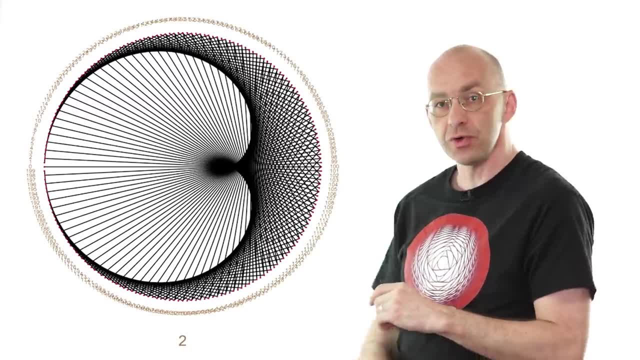 So the number of petals is n minus one, Yeah, n minus one, and it keeps on going like this. so there's a pattern like this: Okay, so let's just start again with two. okay, So that was two times the table. 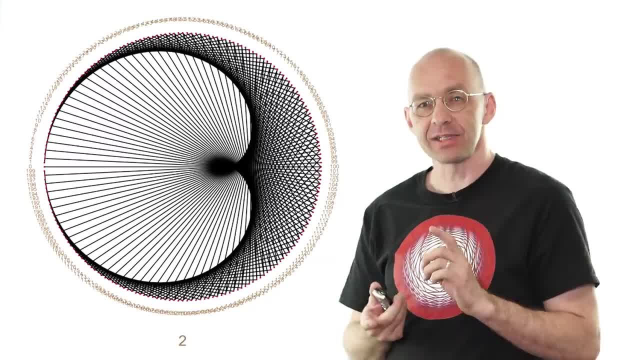 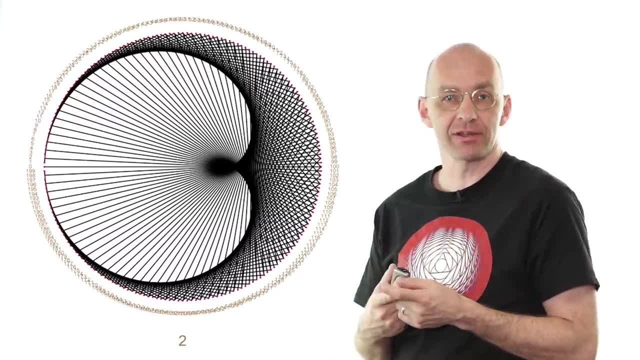 Now one really nice thing to try is actually make the increments not one to three, to four, to five, but actually do smaller increments okay, Or actually do smaller increments okay, Or actually do the transition here continuously. So let's show you if I just do the multiplication. 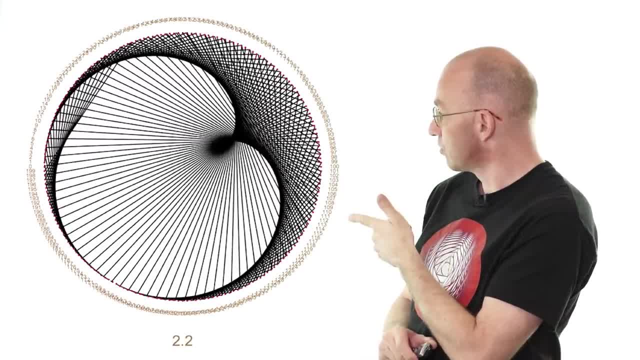 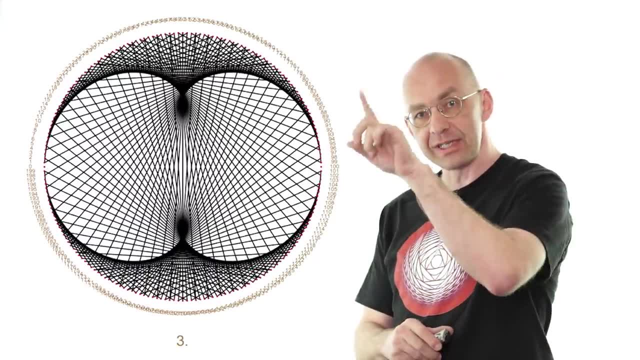 times two point one. what do you get? Two point one, two point two, two point three, two point four, two point five, two point six, two point seven, two point eight, two point nine and three, And you can kind of see how the cardioid turns. 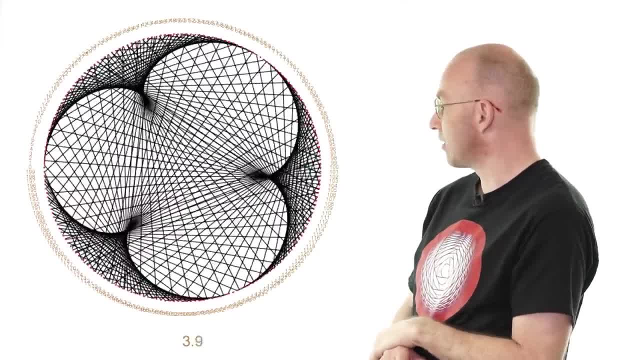 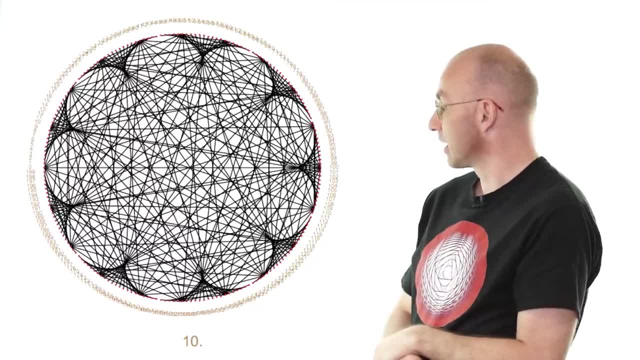 into this nephroid, which is kind of cool, right. And now I just let it go and the numbers are going up and you can see the petals going more and more and more and more right. So it goes continuously. 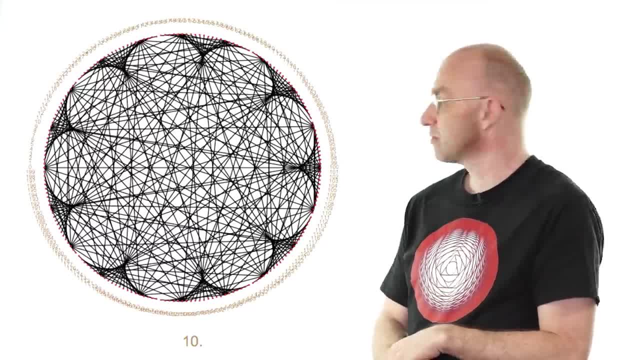 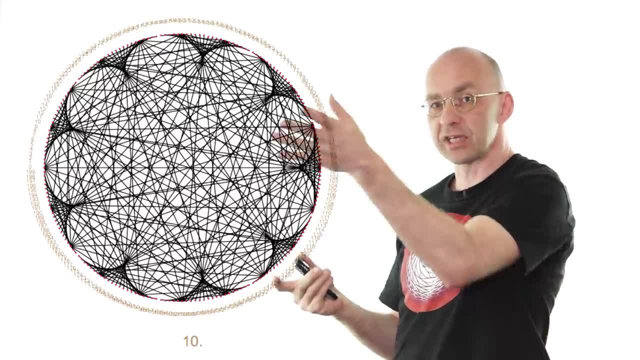 And when you think, well, that's probably what it's going to be. you know, You can also look at this in the Mandelbrot set and you can actually see exactly this sort of pattern here happening in the middle, And if you kind of push the exponent to infinity, 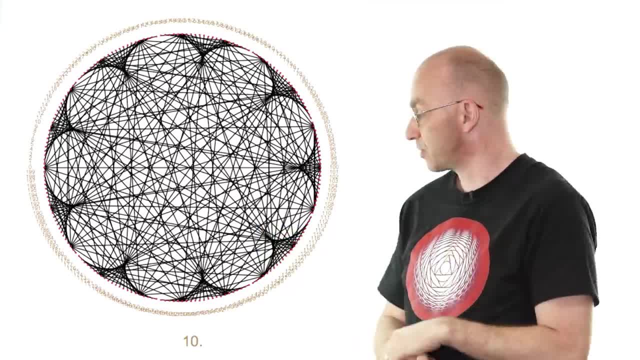 the whole thing kind of turns into one big circle. You know, that's pretty cool, Okay, and that's. you know, I think that's the end of it. but no, no, no, let's just keep going here, all right? 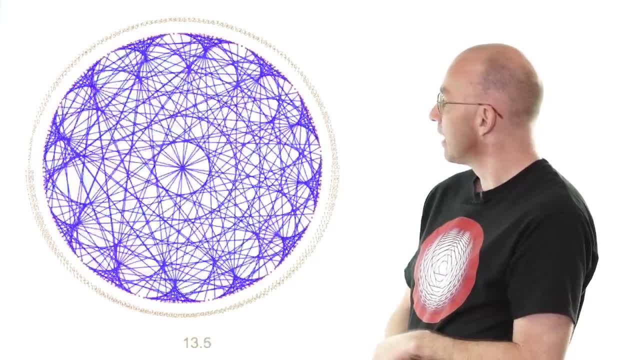 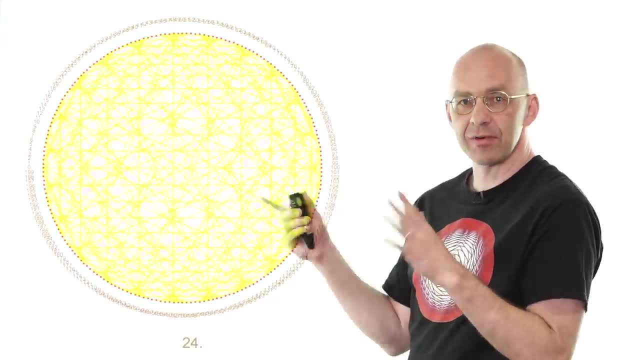 So the petals are pretty much going to go away now. But if you just look at what's happening here, you see there's a lot more. you know structure somehow being hinted at, right? I mean, we're moving very fast at the moment, right? 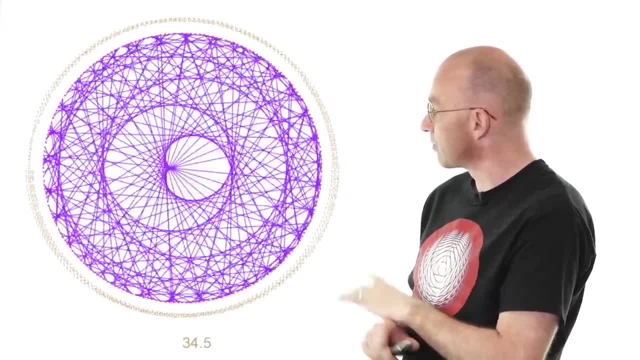 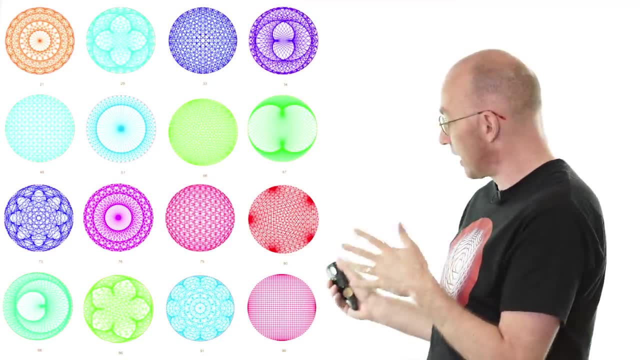 We're moving very fast, But if you actually went through this frame by frame, you would see a lot of really, really nice structure happening And I've highlighted a bit here. So just a few of the frames that you get. You know, some really amazing stuff happening here. 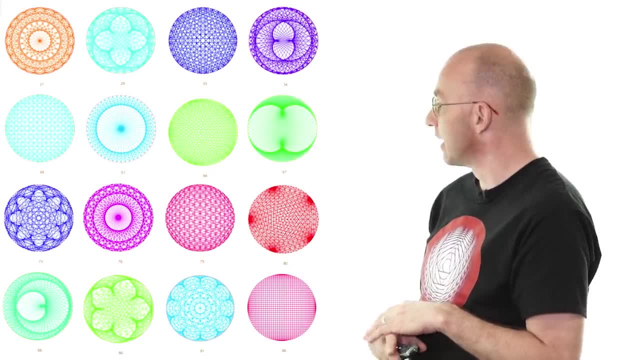 So if you stop at 33, you get this one here. You stop at 34, you get that one here, And there's a couple of other highlights here. There's a lot more. It's just this is how many I could fit here, right. 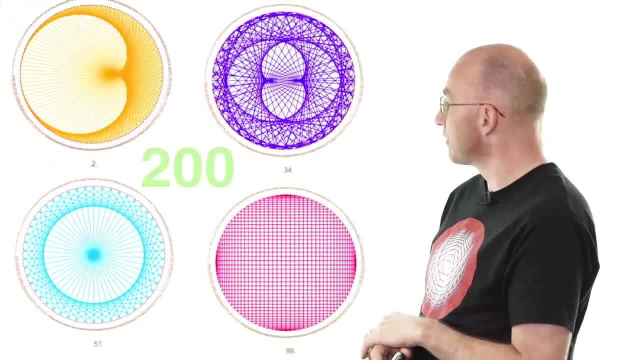 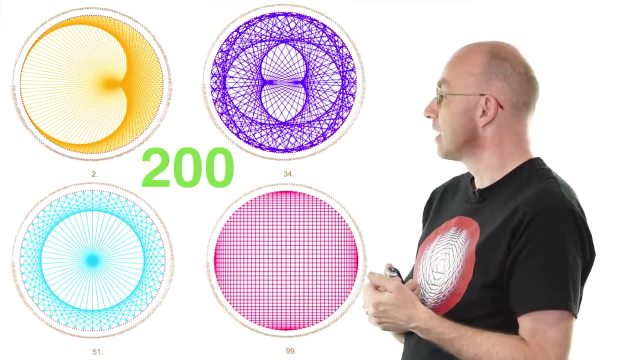 Okay, and maybe have a close look at some of them. okay, So here we've got four. Now, the number that all these correspond to is actually 200, okay, 200.. What we're really doing here has a special name in mathematics, okay. 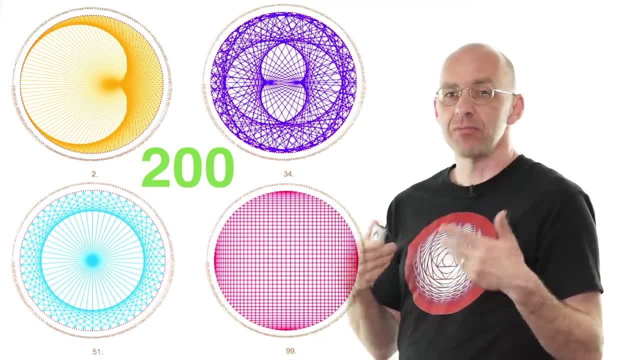 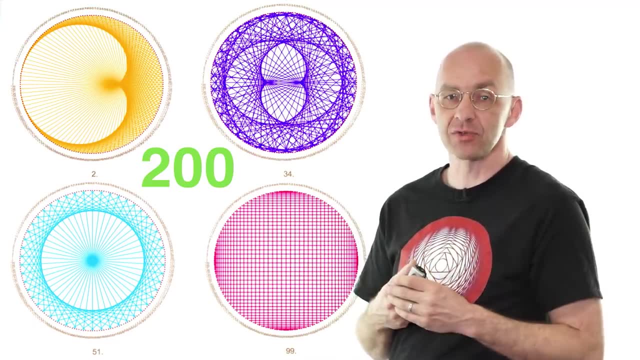 So what we're really doing here is we're doing the times table, modular 200, okay, So it's got a special name. It's actually incredibly important in all sorts of applications to do this sort of modular arithmetic. okay, But anyway, for our purposes, you know. 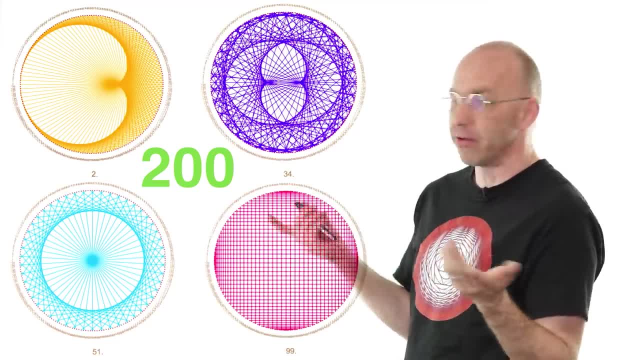 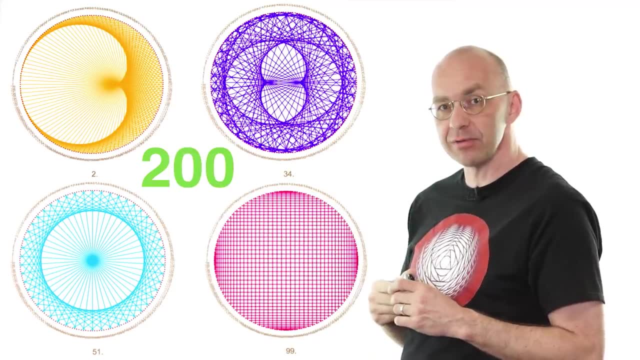 you understand how it's built up And if you know a little bit more, you know a little bit more. Okay, So, for two times table, we get the cardoid. For the 34 times table- modular 200, we get this guy here. 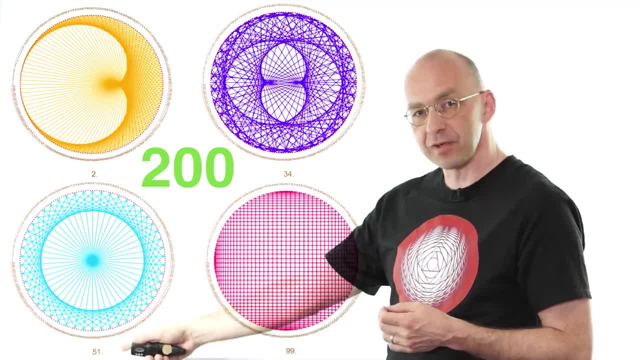 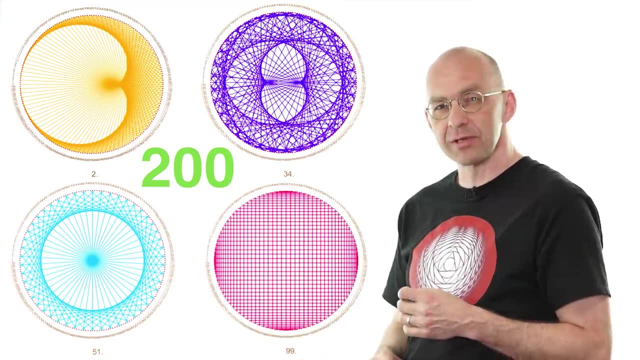 And then some other things, interesting things happen. So for example, if you multiply by 51, we get this guy here, And if you multiply by 99, we get that guy here. And obviously I mean, if you just look at the two numbers here below- 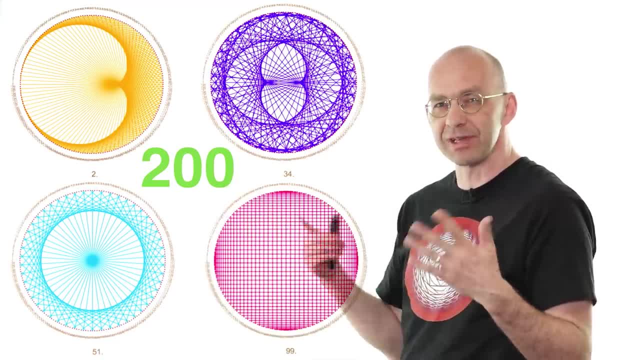 you know, 51 is pretty close to, you know, 1 fourth of 200. So it must have something to do with that. 99 is pretty close to 1 half of 200. It must have something to do with that, right. 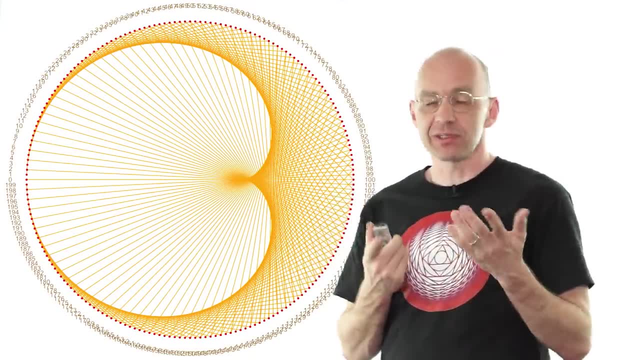 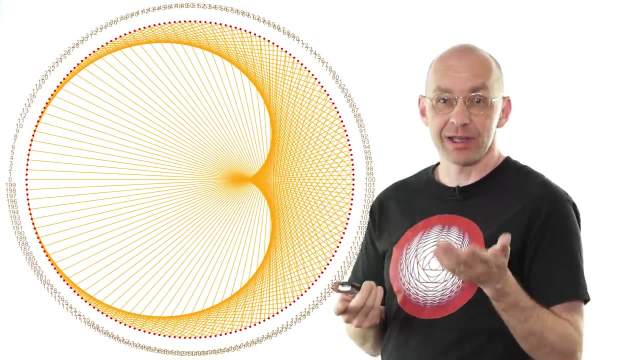 Okay, Now I really wanted to explain something. I really want to explain where this one here comes from. And well, I mean, the first time I saw this I was pretty surprised, like pretty much everybody, I see. But then I remembered something. 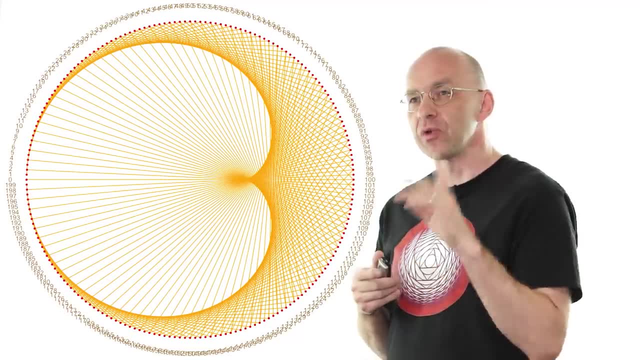 I had seen the cardoid before in you know many, many different guises, And in one particular one that I was familiar with I could see where the connection is, And I just want to tell you about that one. okay. 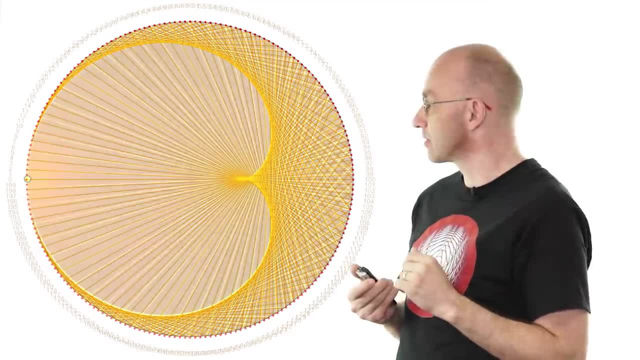 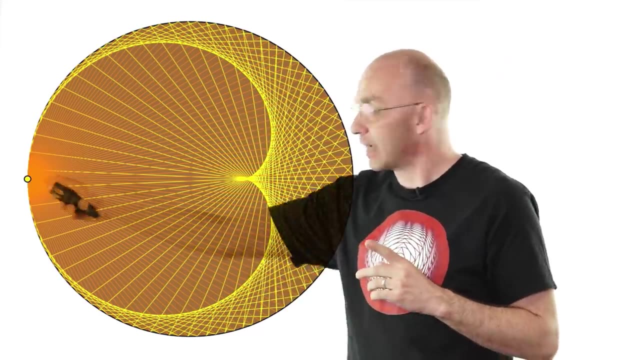 And it's got to do with this- light rays bouncing around. It's a little bit different from what we had before, okay? So basically we've got a circle here And then we've got a light source right over on that side, right? 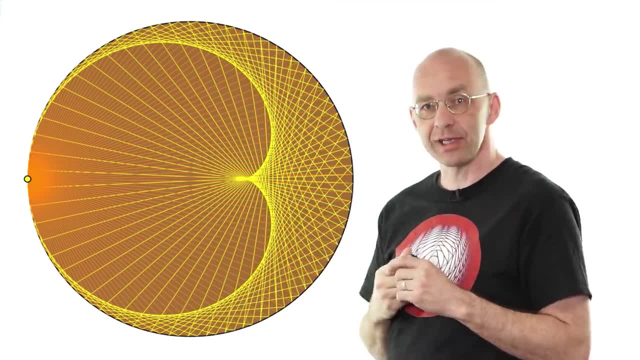 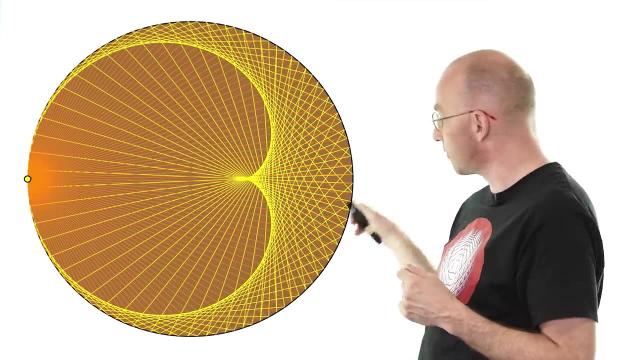 And that circle kind of reflects the light right. So we switch on the light over there And then, well, what happens? Well, light rays kind of emanate in all kinds of directions, get reflected off the circle right. 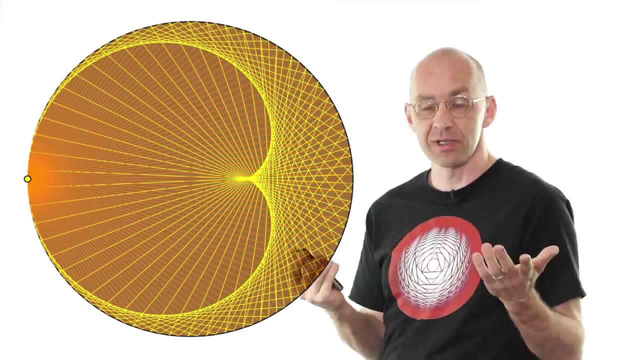 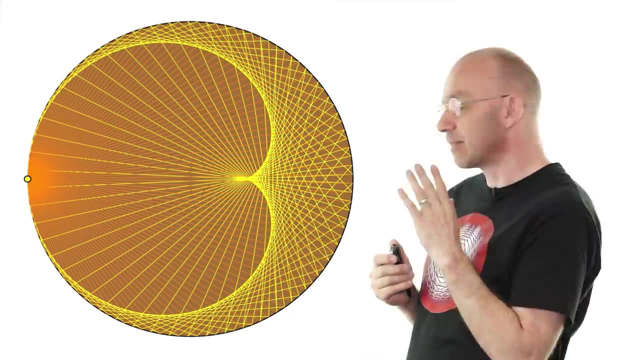 Bounce around and you kind of see this pattern here emerging. the cardoid: Yeah, I knew this one. I had actually calculated the curve you know from this description at some point in university. okay, Then they can actually really see very easily. 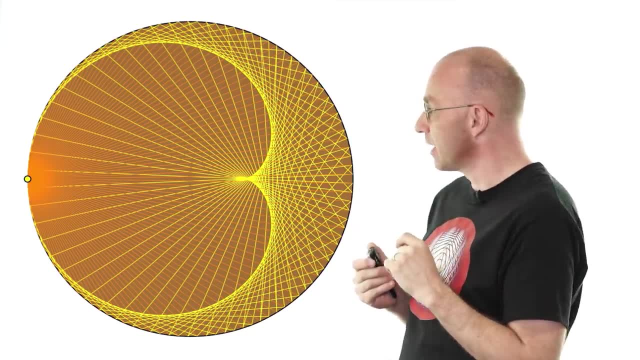 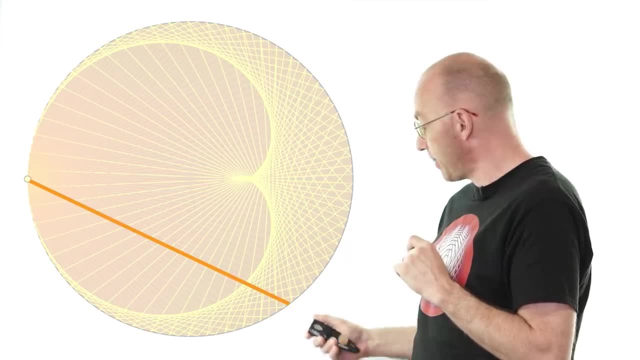 why the cardoid comes up in the two times table And I just want to show you, okay. So let's just highlight: like one of those rays coming out, It kind of hits the wall here, okay, And then it gets reflected at the same angle as it comes in, right? 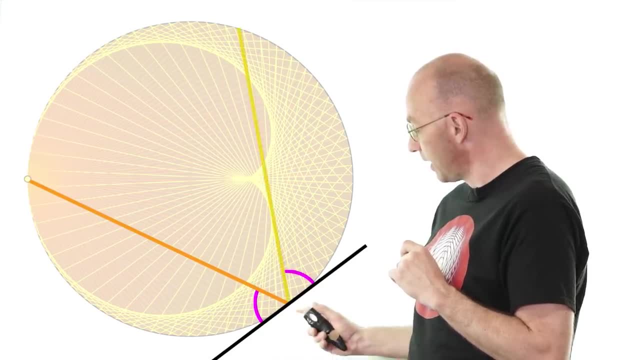 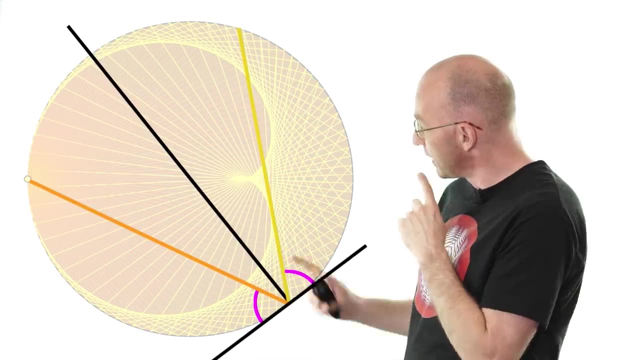 So this angle here that you see here is the same as there, right, And you can see it kind of goes like that: Okay, so what does that tell us now? Well, if we kind of put this line here in the middle, 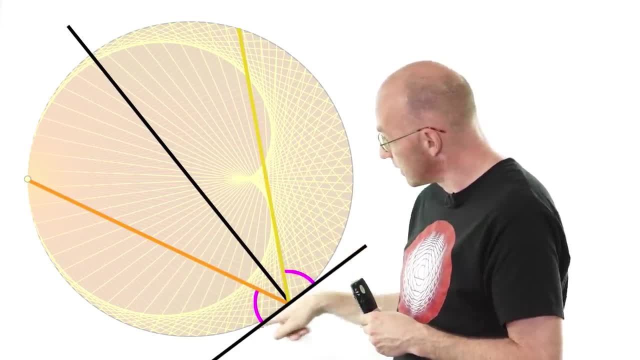 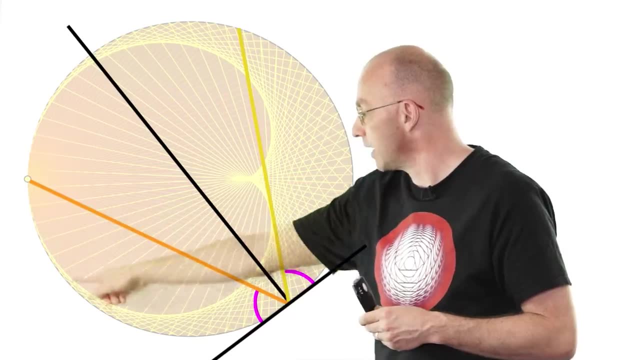 it means that this side really flips over to that side here, which means that this segment here in particular is exactly as long as that one here, right? So if I travel from this light bulb to this point and then from this point to that point, 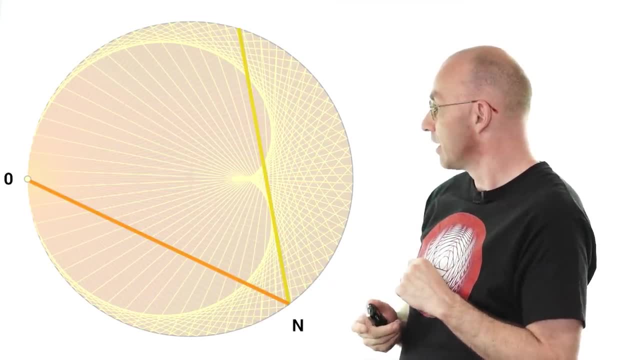 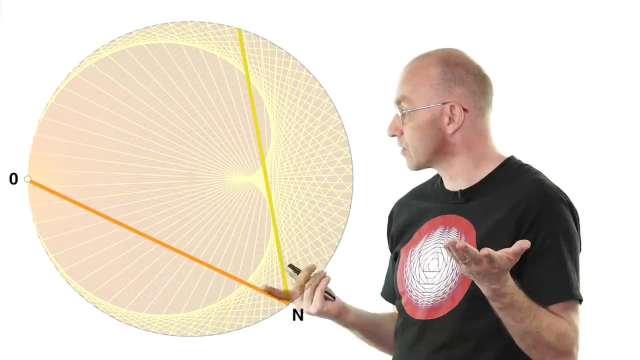 it's exactly the same distance. okay, So that's going to be important. So let's make this zero. Let's call this n, So what's 2n? then? right, So to get 2n, what we have to do is we have to measure this distance here. 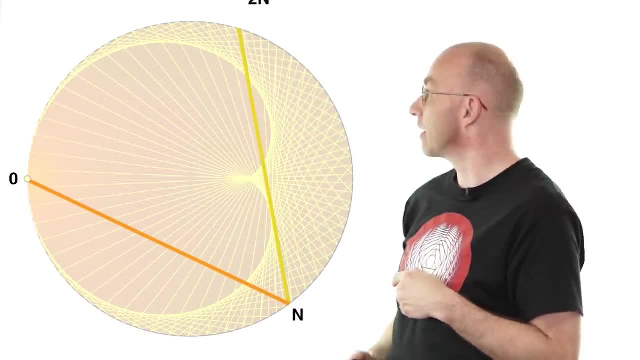 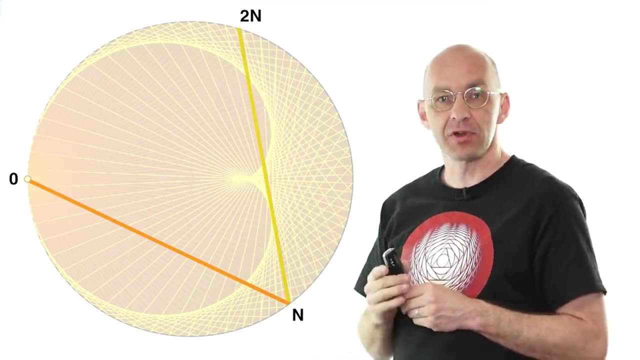 and then we have to measure it again. Where do we get Right up there? And so it's pretty clear that when you do the two times thing, you get that reflected ray, you know, in the picture. Just to finish off, I'm going to show you a little bit of a movie. 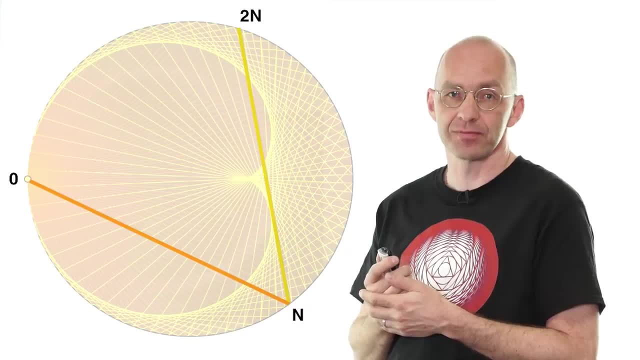 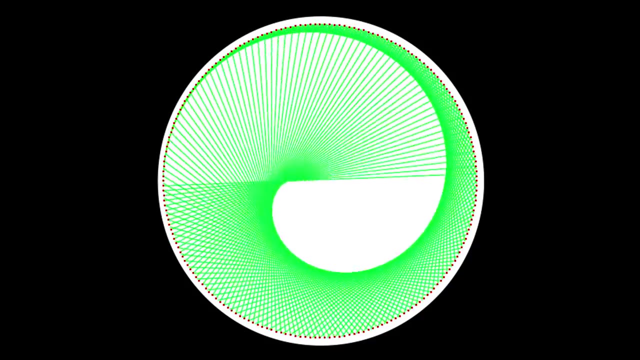 of all the stuff evolving a little bit slower than what we had before. So I have a lot of details here. So what you're going to do is go back and see what I just didn't. So I have to go over it again. 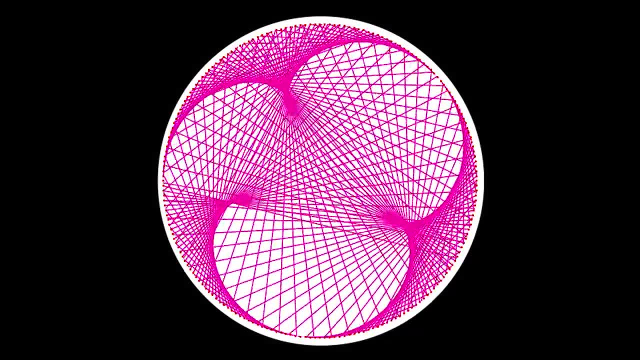 I'm going to go over this dot here And then I'm going to edit this just a little bit. So what you're basically going to do is you're going to go and change the position of this dot here. it's going to change this dot. 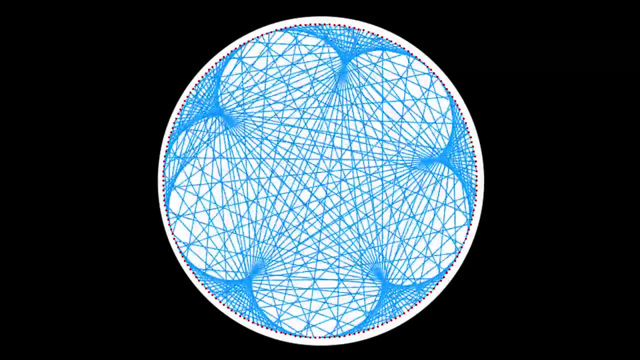 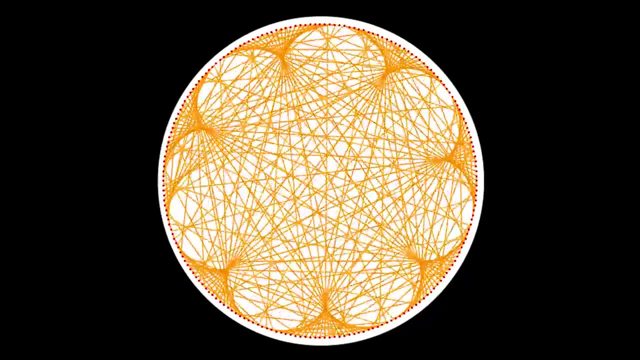 it's going to change the position of this dot here. So right now I'm going to do a table, So what we have to do is you're going to have to get them all here And you're going to see the distance here. Thank you, Thank you. 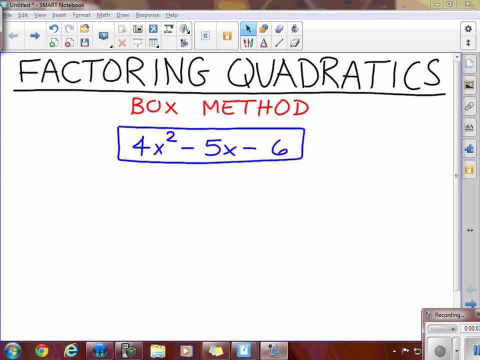 This example is going to illustrate how to factor a quadratic using the box method. It doesn't matter which method we use to factor a quadratic. we always have to consider the quadratic and look for any greatest common factors within it. So here's my quadratic. 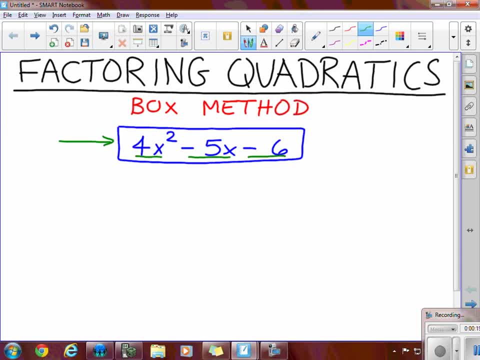 I have a 4x squared, a negative 5x and a minus 6.. None of the numbers 4,, 5, or 6, have any common factors, and the first two terms have x's in them. The last one does not.